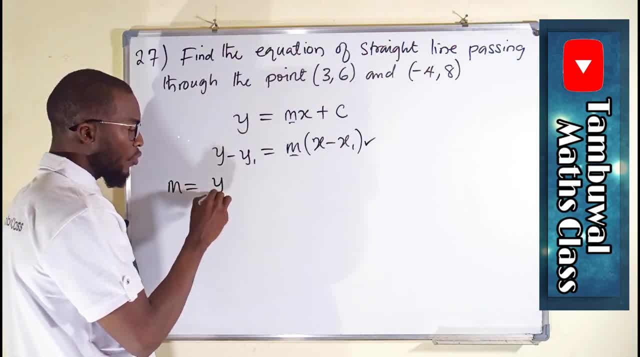 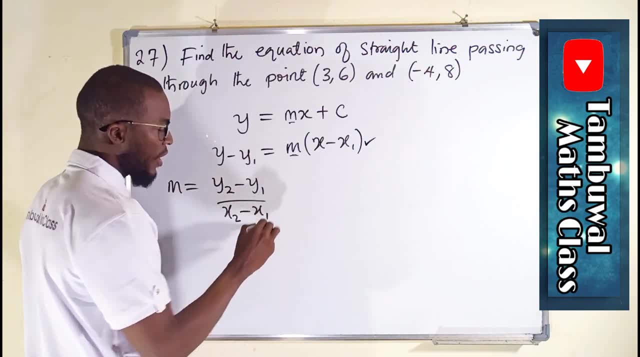 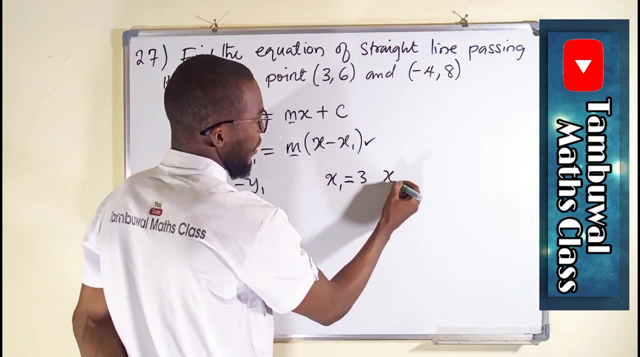 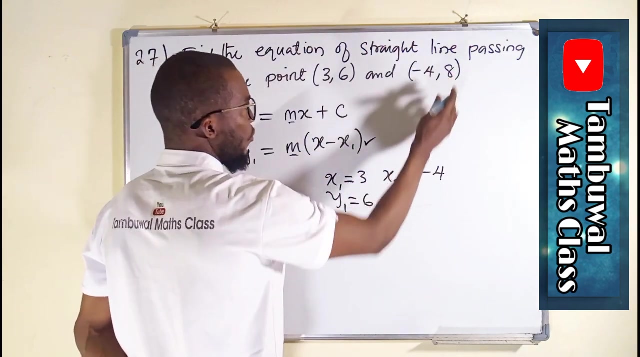 the m is equal to y 2 minus y 1, divided by x 2 minus x 1. from this point you can see that x 1 is equal to 3 and x 2 is equal to negative 4, y 1 is equal to 6 and y 2 is equal to 8. so we can substitute here: 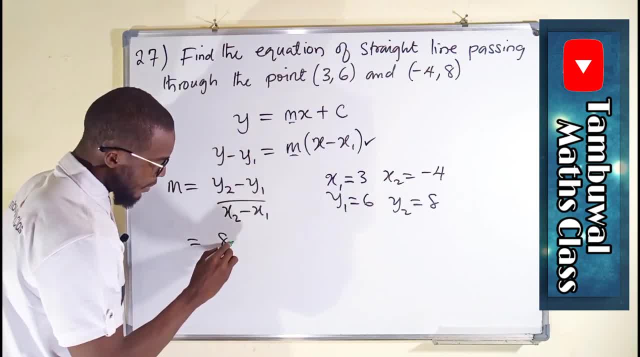 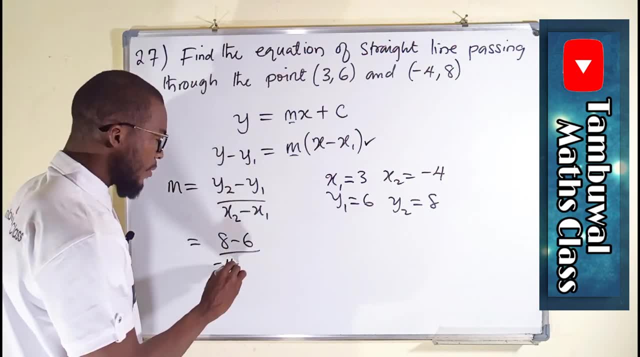 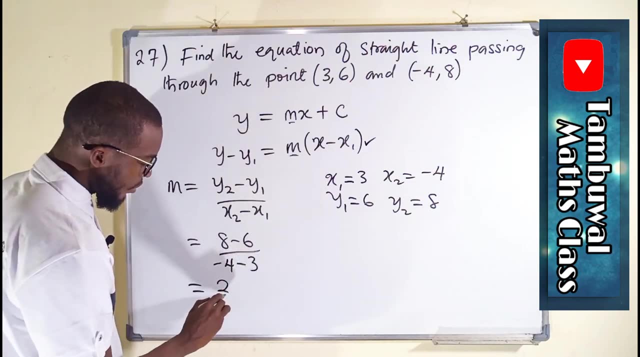 this is equal to y 2. we have it as 8 minus y 1, which we have as 6 divided by x 2, which is negative, 4 minus x 1, which is 3.. this is equal to this minus this is 2 over. 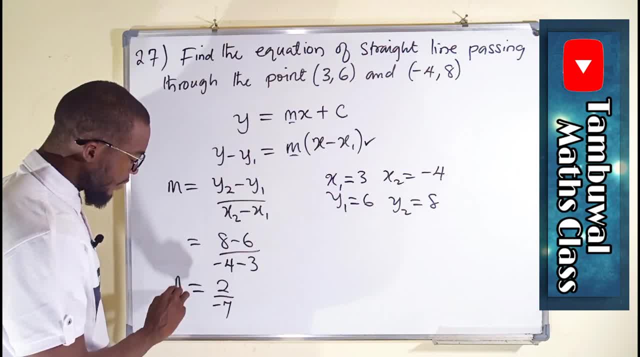 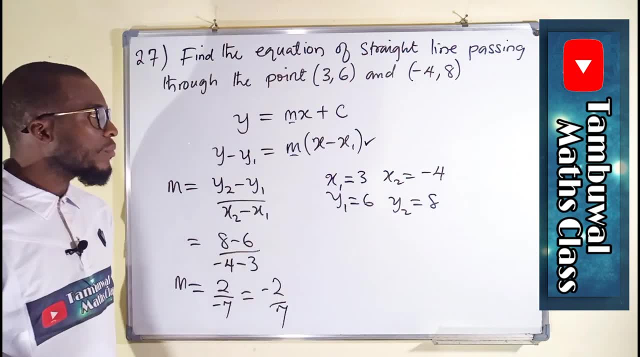 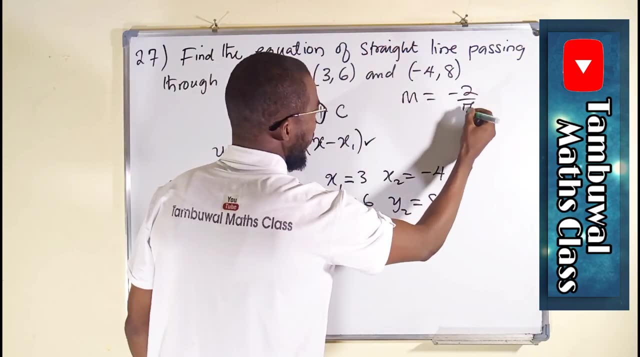 minus 3 is minus 7, and hence our slope, m is equal to minus 2 over 7.. so now let us keep that aside. m is equal to minus 2 over 7.. so now let us use this slope to find our equation. 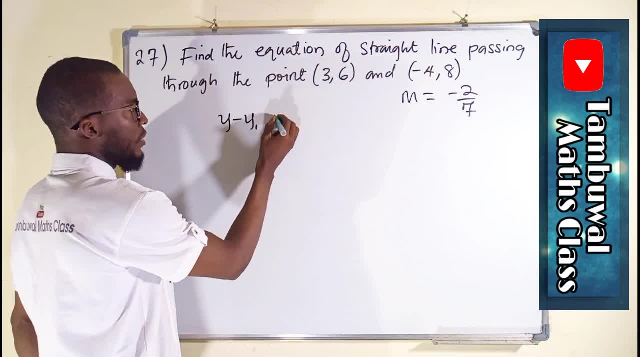 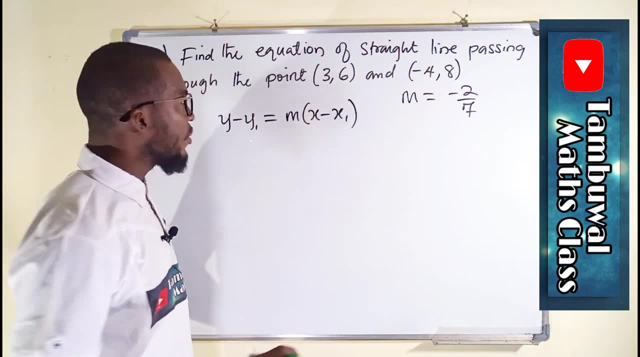 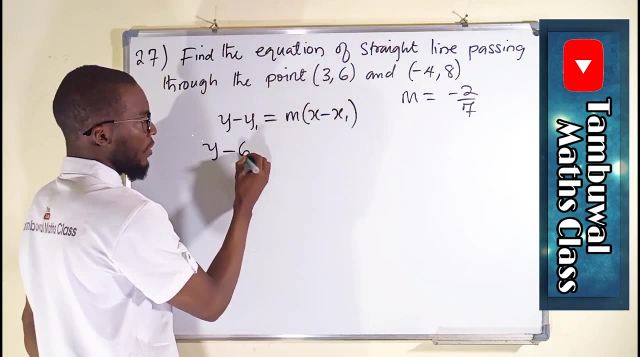 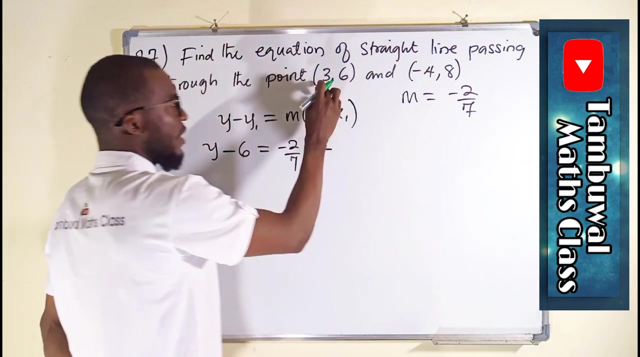 we say that y minus y 1 equals m. multiplied by x minus x 1 is our linear equation. y is still y minus y 1. this is our y 1, which is 6 equals m, is negative 2 over 7 times x minus x 1 and x 1 is 3.. 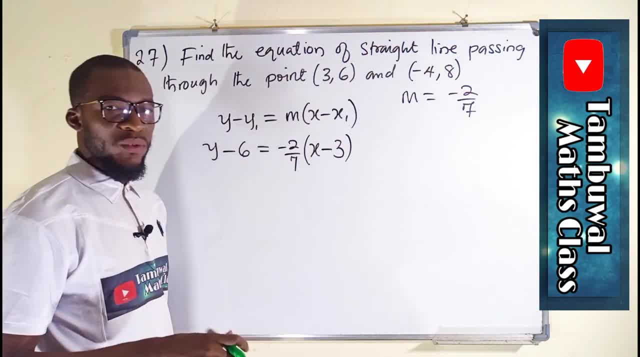 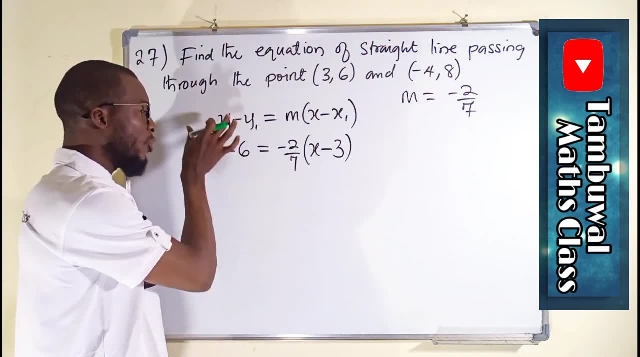 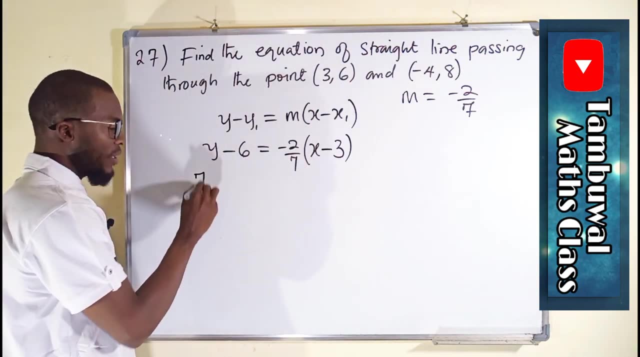 remember i told you to deal with an algebraic equation that contain fraction. as simple as that. you need to eliminate the fraction first. to do so, we have to multiply both sides by this 7 in order to eliminate it out. so 7 times Y is 7Y. 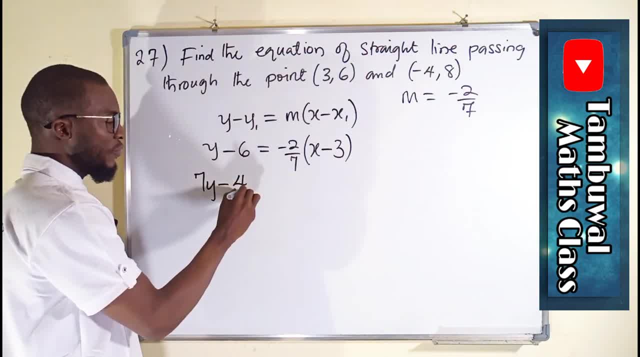 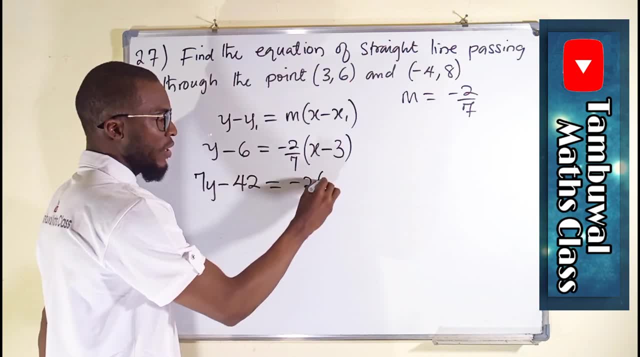 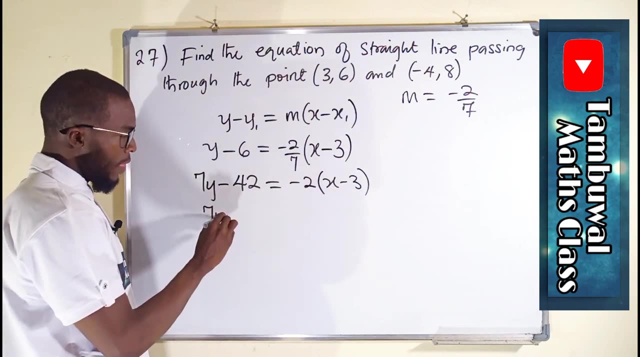 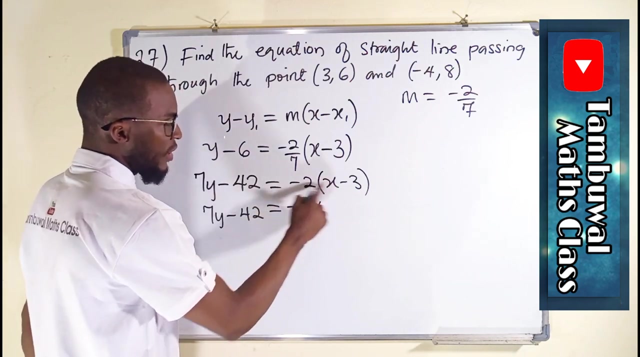 minus 7 times 6 is 42 and this is equal to. if you multiply this by 7, they will cancel out, leaving minus 2 times X minus 3. you can expand this so we have 7Y minus 42 equals this time. this is negative, 2X negative. negative. positive, 2. 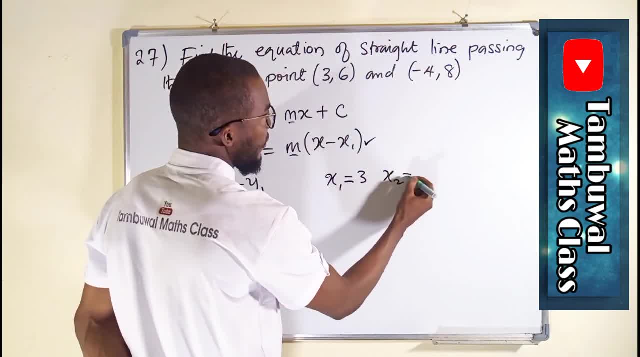 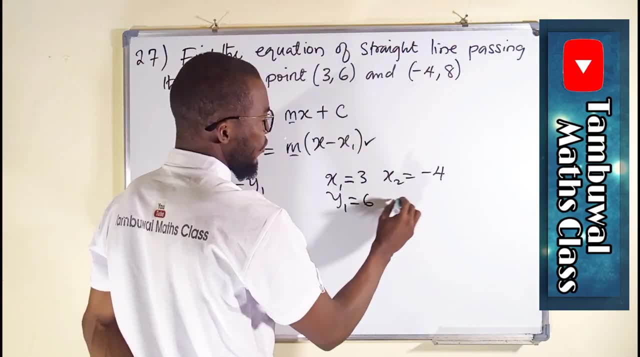 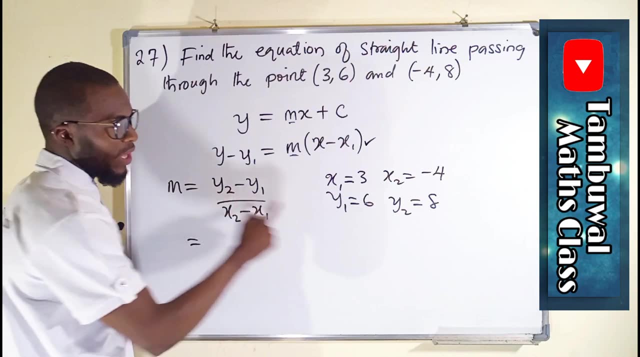 x 1 is equal to 3 and x 2 is equal to negative 4, y 1 is equal to 6 and y 2 is equal to 8, so we can substitute here: this is equal to y 2, we have it as 8 minus y 1, which we have as 6. 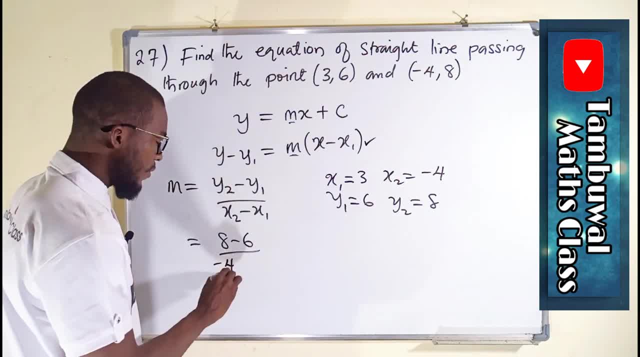 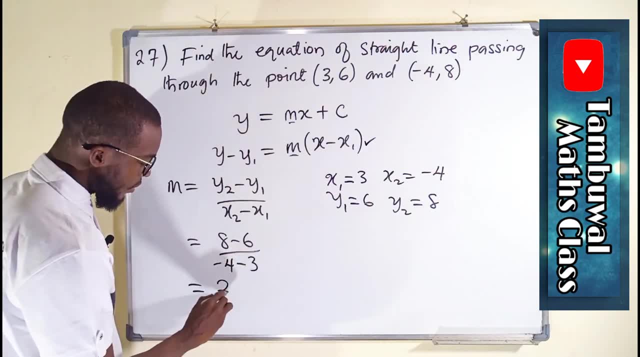 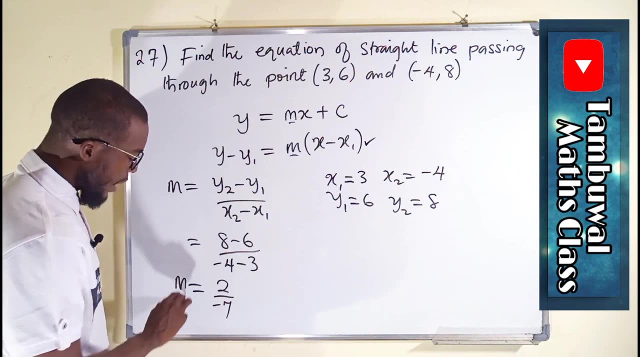 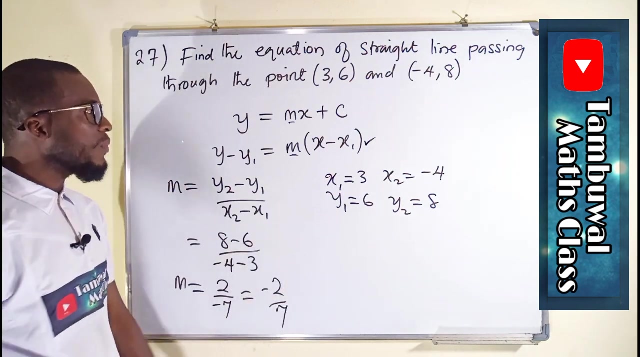 divided by x 2, which is negative, 4 minus x 1, which is 3, this is equal to this minus. this is 2 over minus 4. minus 3 is minus 7, and hence our slope m is equal to minus 2 over 7.. so now, let us keep that aside. m is equal to minus 2 over 7.. 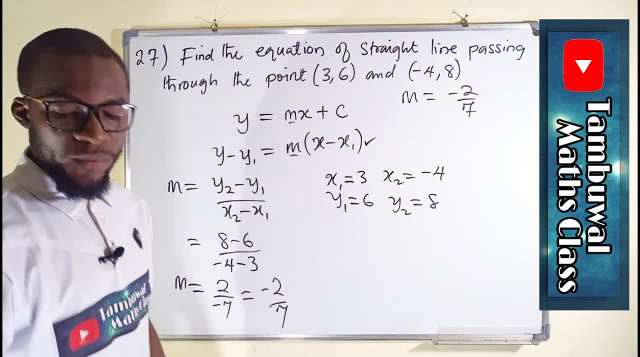 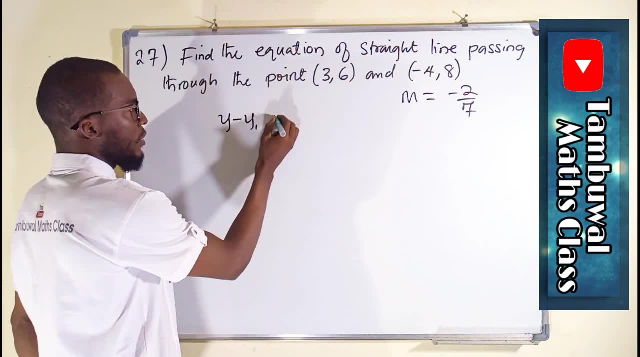 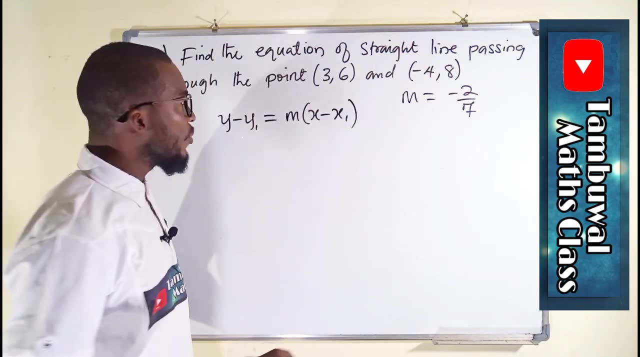 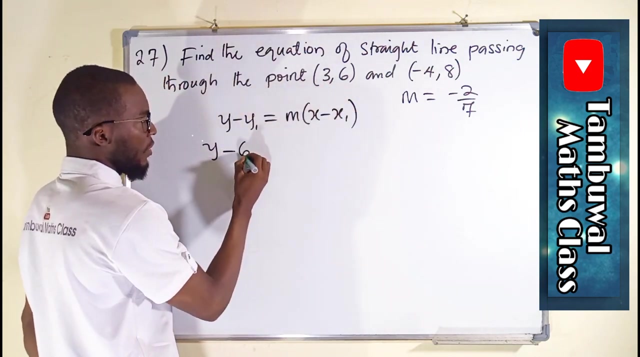 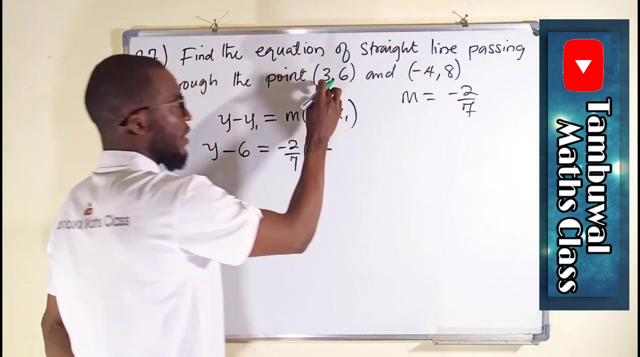 so now let us use this slope to find our equation. we say that y minus y 1 equals m. multiplied by x minus x 1 is our linear equation. y is still y minus y 1. this is our y 1, which is 6 equals m, is negative 2 over 7 times x minus x 1 and x 1 is 3.. 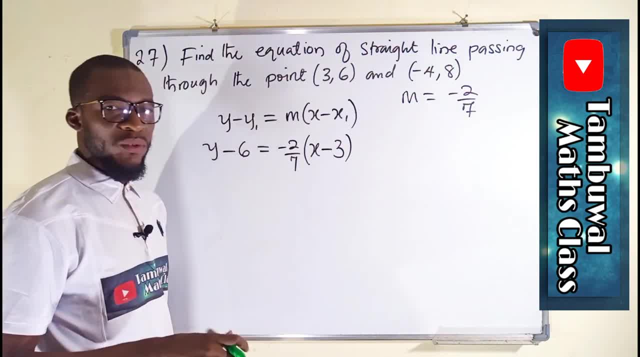 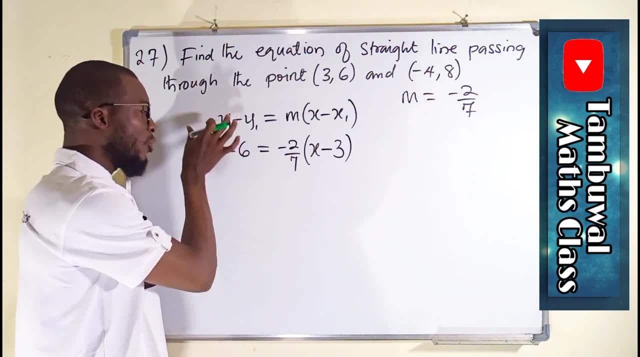 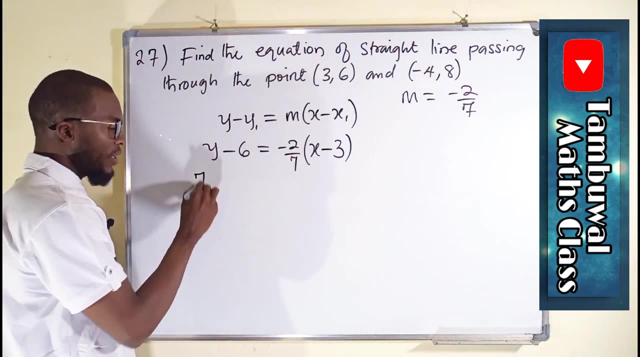 remember i told you to deal with an algebraic equation that contain fraction. as simple as that. you need to eliminate the fraction first. to do so, we have to multiply both sides by this 7 in order to eliminate it out. so 7 times y is 7y. 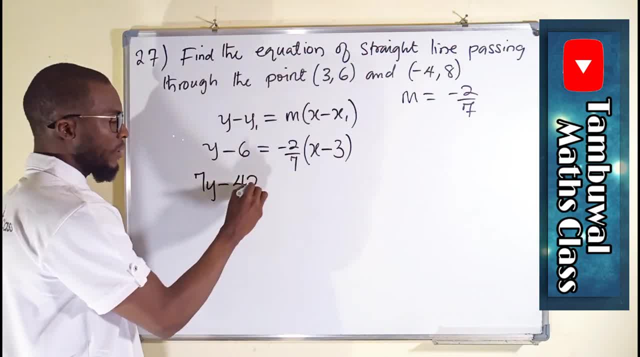 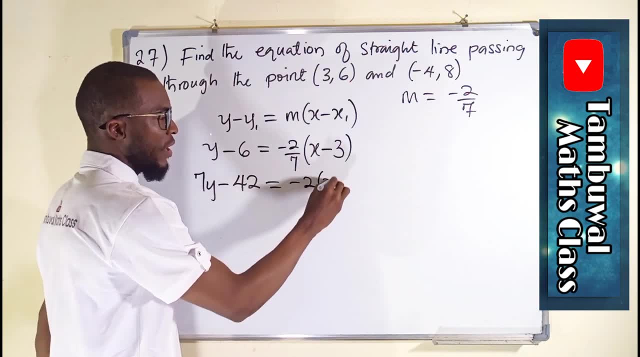 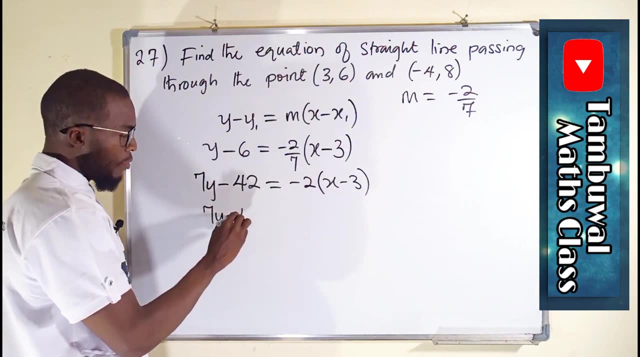 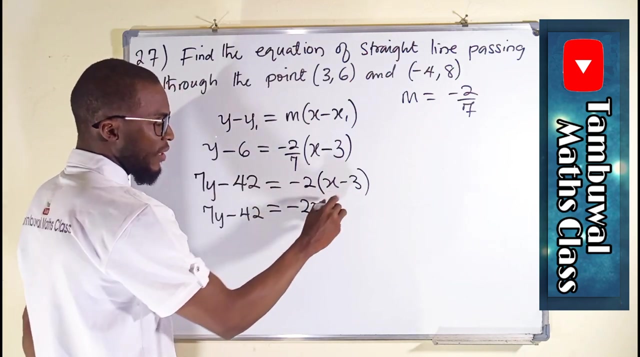 minus 7 times 6 is 42 and this is equal to. if you multiply this by 7, they will cancel out 11 minus 2 times x minus 3.. you can expand this so we have 7y minus 42 equals. this time. this is negative, 2x negative. negative, positive 2 times 3 is 6.. 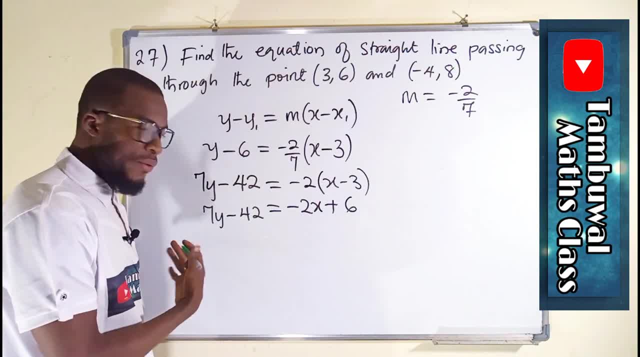 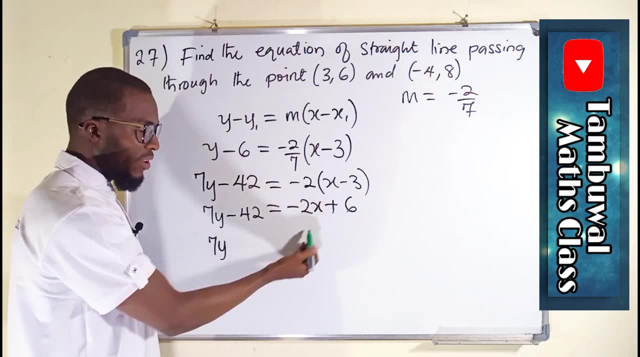 now we can bring those with variables to the left and thus constant to the right. we have 7y here. we have minus 2x to the right. if it crosses over, it becomes positive: 2x, 2x, 2x, 2x, 2x.